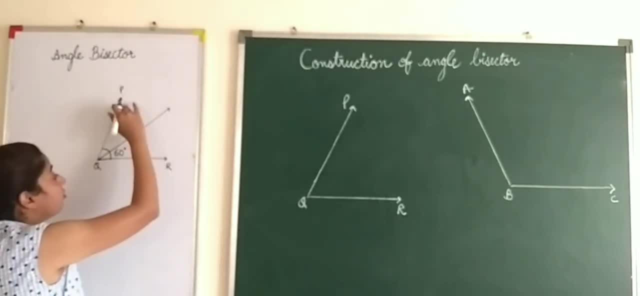 draw a bisector. So the bisector is the ray which divides the given angle into two equal halves. Now suppose this is S, So I can say angle PQS, that is, this angle is 30 degree and angle SQR, that is, this angle is again 30 degree. So what this ray is doing, This ray, QS, has divided the 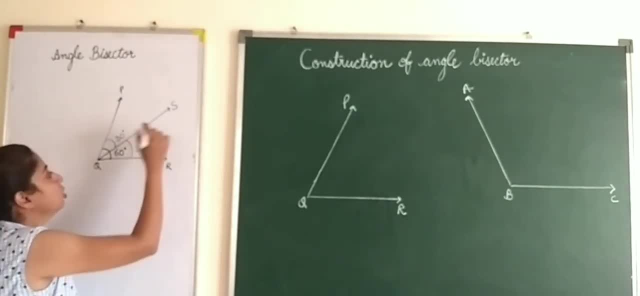 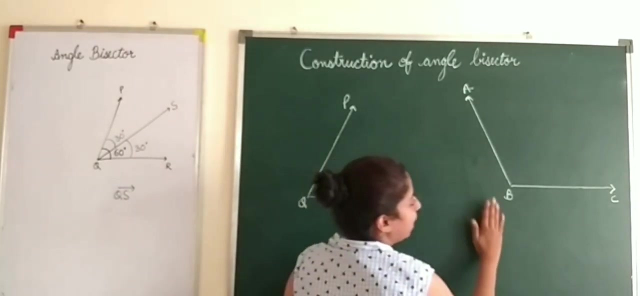 angle 60 degree angle into 30 degree and 30 degree, So the ray QS. the ray QS is the angle bisector of angle PQR. Now say, here I have drawn two angles: angle PQR, which is an acute angle, and angle ABC, which is an obtuse angle. Now let me tell you how to construct the 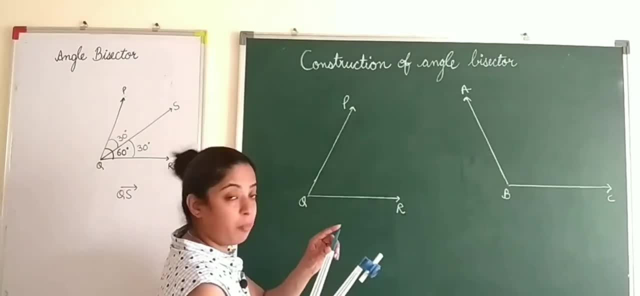 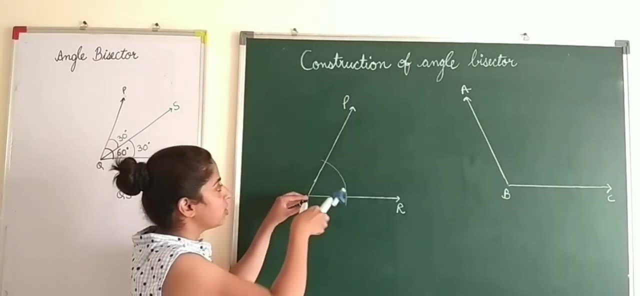 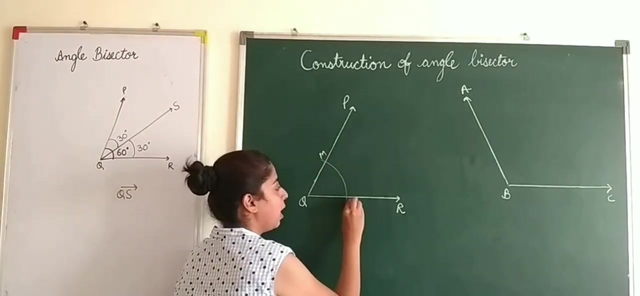 angle bisector. For this, take your compass, keep the point of your compass on the vertex of the angle that you want to divide. Then draw an arc such that it cuts both the arm at two different points. You can name these points: M and N. You can change this measurement now. Now keeping the 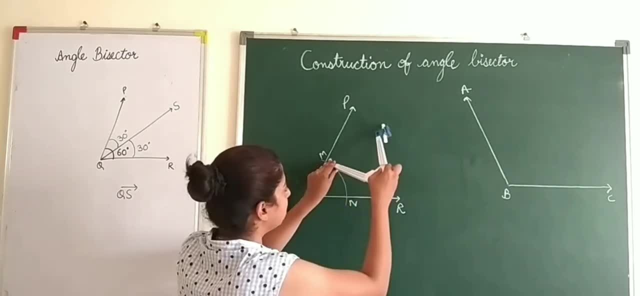 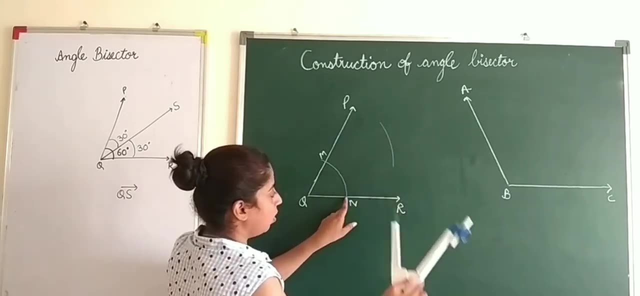 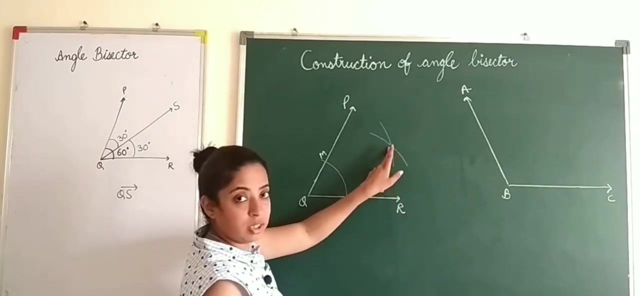 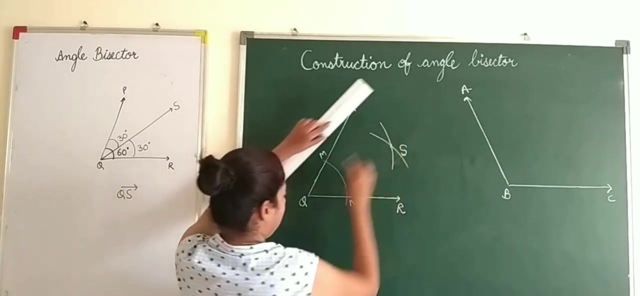 point on M. So, keeping M as the center, you draw an arc Now, keeping the same radius. keep the point on N, Okay. So taking N as a radius, you will again cut the previous arc. So you have got this. Give any name to this point, Say S- Okay, And then you join this point: S and Q. 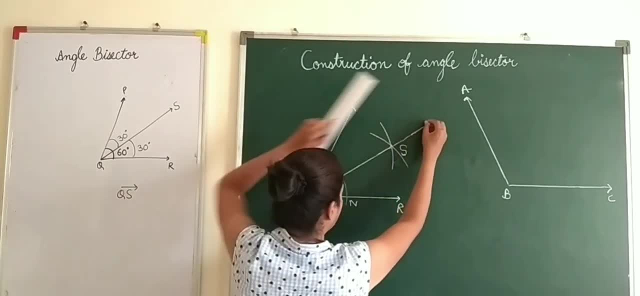 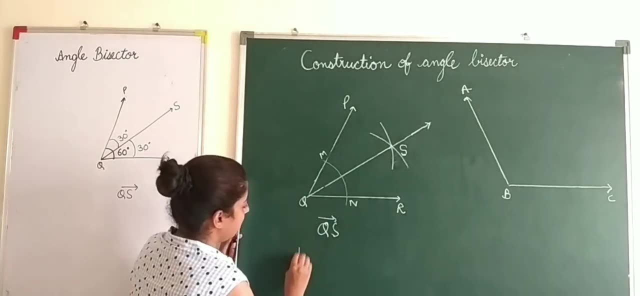 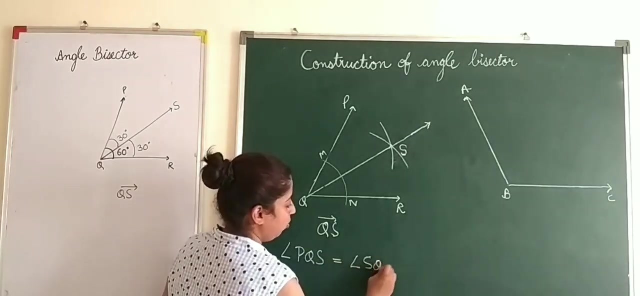 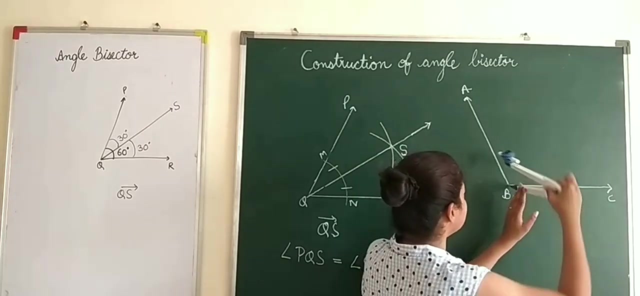 You can extend this. So this ray QS, is the required bisector. Okay, So you can say now, angle PQS is equal to angle SQR. So this ray has divided this angle into two equal halves. Now let us see this angle ABC. We follow the same method, Keeping B as